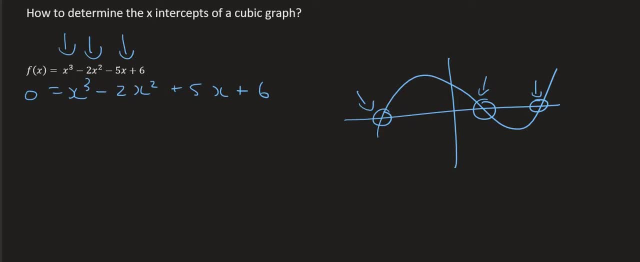 until you get a value of zero. Now the numbers that you want to choose will be one, two, three minus one, minus two and minus three, One of those numbers. what you do is you keep plugging in those x-values into this equation and you keep going until you get a zero. 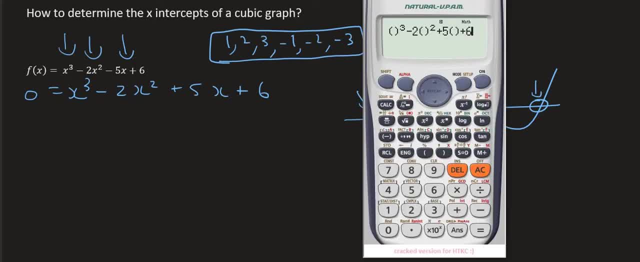 So what I mean is the following: So what I like to do is I make a little template for myself, like that on the calculator, and then we can just plug in different values. So we could plug in a value of one, for example, and then we get an answer of ten, and that's not what we want. 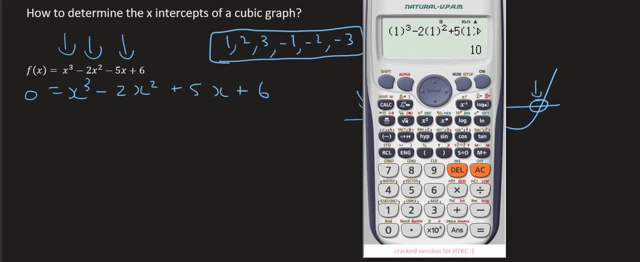 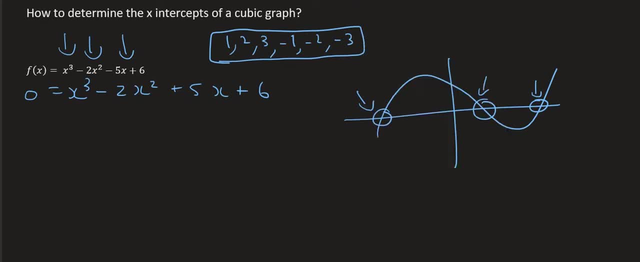 okay, We're looking for a number. We want to get an answer of zero. Oh, I just realized I've made a mistake and sorry for any of you at home who picked that up Over here. this was a minus and then I went and made it a plus, So on the calculator I've also got it as a plus and 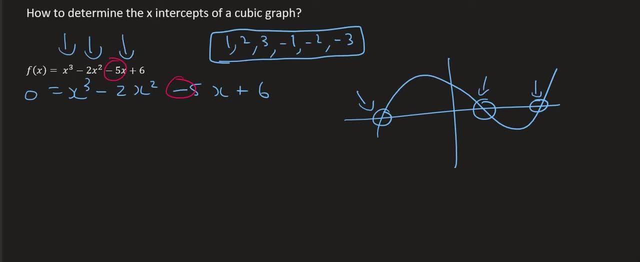 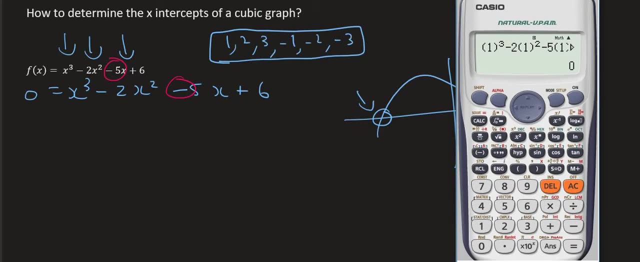 that's why it's not working. So this should be a negative. There we go. and then I just need to fix the calculator and then if we say equals, we get a zero. There we go. So I've made a small little mistake. So the x-value of one makes the answer zero. So 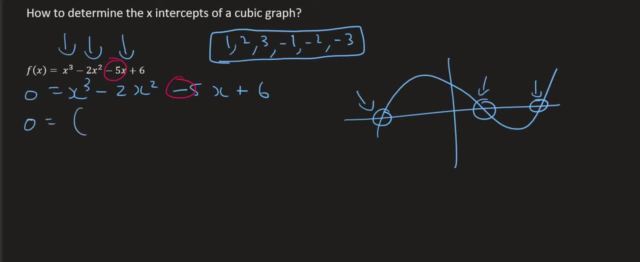 what you do- and you must remember this- is you then make a bracket that will then say x minus one, because, remember, if x equals to one is one of the factors- then you would say x minus one for your first bracket, and then we're going to have one big bracket left over, and then, on the inside, 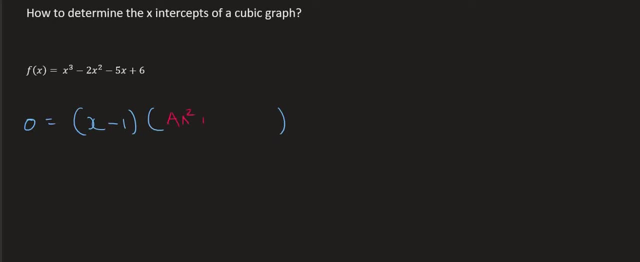 of this bracket. it'll be some type of trinomial, So I'm just going to call it ax squared plus bx plus c. So if you had to multiply these two together again, you would obviously have to get the original expression, and that's going to help us to work out what a, b and c would be. So if you had to, 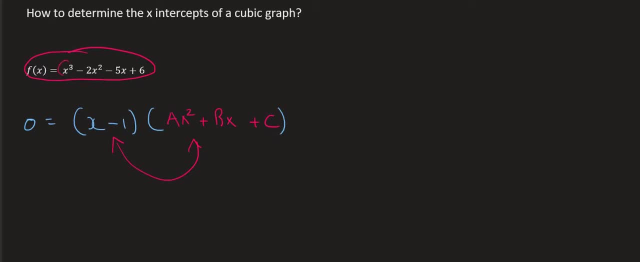 multiply these two brackets together. where would you get x to the power of three? Well, that would only happen in one place. That would be when you multiply this x and this ax squared. Okay, now we know that the original expression, the number in front of the x cubed, is a one. So we know that a. 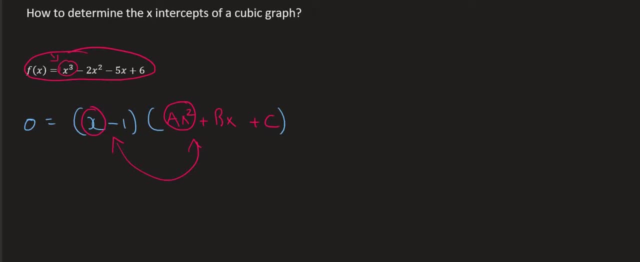 would then have to be one, So that when you multiply those two together you still get x to the power of three. If, for example, the number in front of this x cubed was a two, then this a value would have to be a two, But in this case it's just going to be a one. The next place to check is if 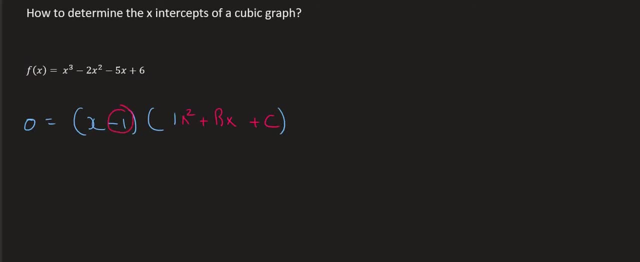 you have to multiply this part. or let me first ask you: where would, if you had to multiply these two brackets together? where would you get a constant? Remember, a constant is something that doesn't have an x in it. Well, that would only be if you multiply this minus one and this c and together. 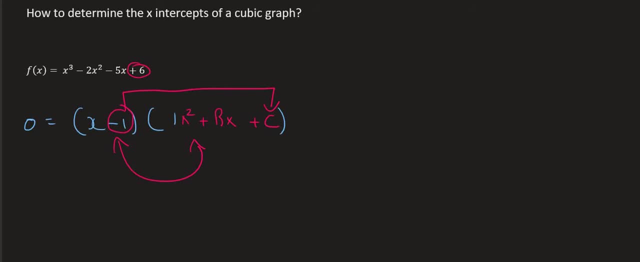 that should give us positive six. So all we're doing in this technique, guys, is we are looking at these two brackets and seeing what the a, b and c would have to be so that we would get back to the original. So we know that minus one times by minus six would give us positive six. 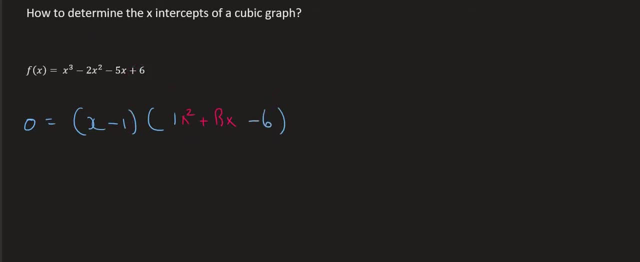 So c is going to be minus six. Now to find b. it's a little more complicated. What you need to do is choose whether you would like to look at the x squares or if you would like to look at the x's. It's your choice. you will get the same answer. So I'm just going to choose the x squares. 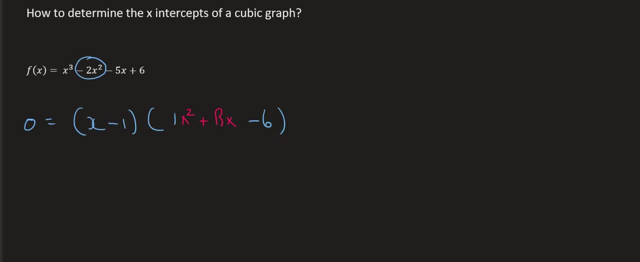 So we know that the x squares should equal minus two. So where would you get an x squared if you multiply these two brackets together? It's going to happen Twice. So it's going to be when you multiply this one and that one that's going to give you an x. 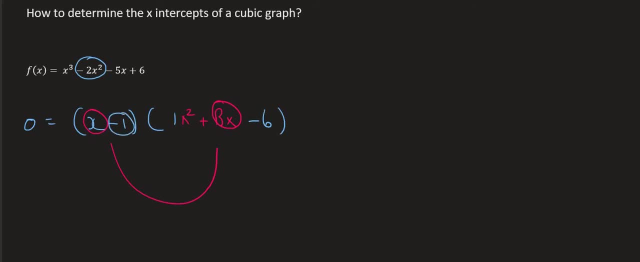 squared, and then it's also going to happen when you multiply this one and this one, So we can set up a little equation. We want the answer to be equal to minus two x squared. That's what we can see there, and so that's going to be the combination of this one times by that one, which is b x squared. 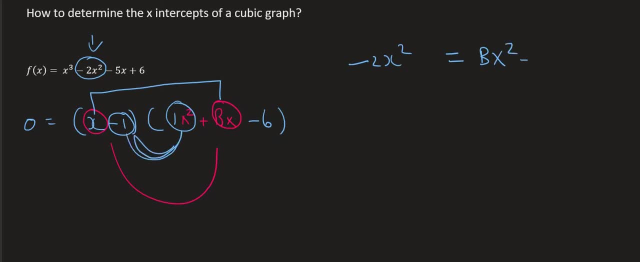 and then this one times by that one, which is going to be minus one, x squared, So that's going to be x squared. You can then ignore the x squares, and so we end up with: minus two is equal to b minus one, and so b is going to be equal to minus one. There we go. So now to find the other two, x.